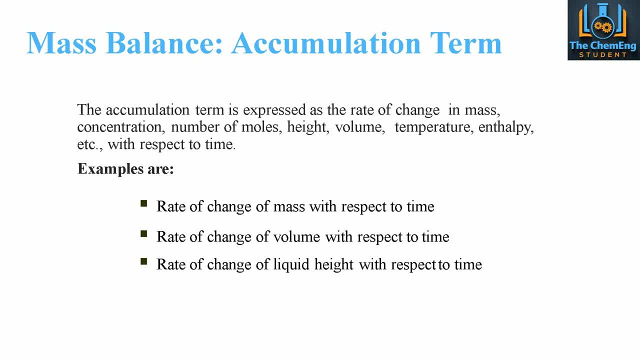 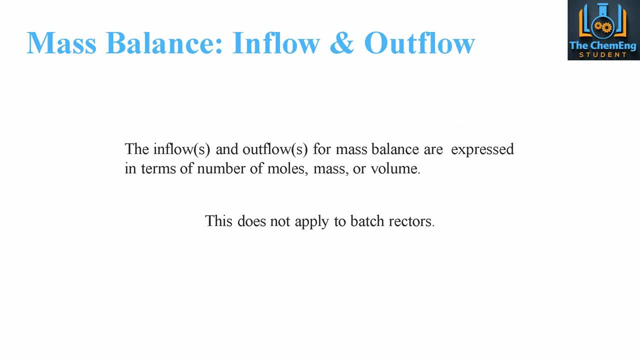 variations that we can have. All are with respect to time. Now the in and out flow is that are expressed in terms of the number of moles, the mass or the volume which comes into the system and leaves the system. Now, for batch reactors, this doesn't apply. This would only apply for 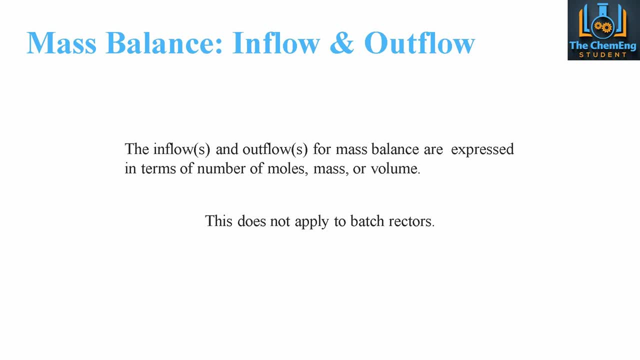 CSTRs and plug flow reactors. Also, if you have fixed bed catalytic reactors with an in and an out flow as well. Now, one thing to note is that when we deal with these kind of equations, if we have reactions taking place, so if we have a reacting system, then we have to do everything. 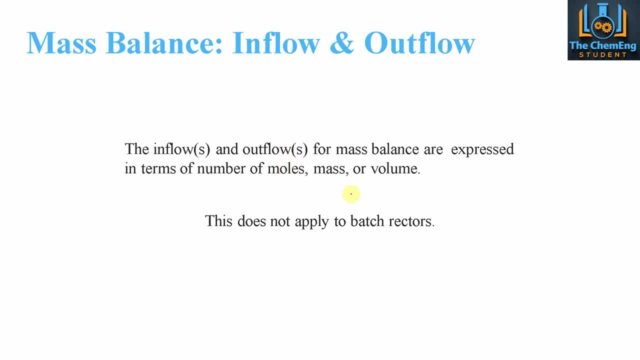 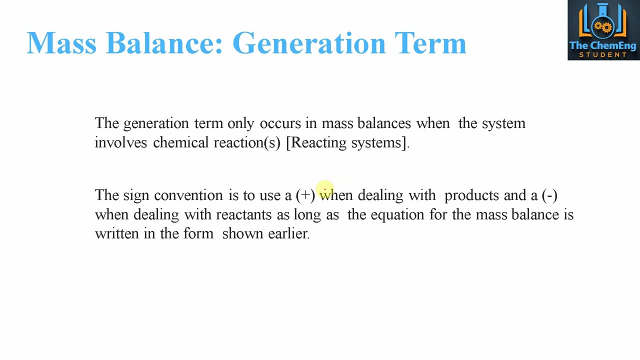 in terms of moles, because moles is the thing that we can relate each component to. We can't relate it in terms of mass, so we have to do it in terms of moles. Now the generation term will only occur when a reaction is involved, ie reacting systems. Now the sign convention here is: we've seen that: 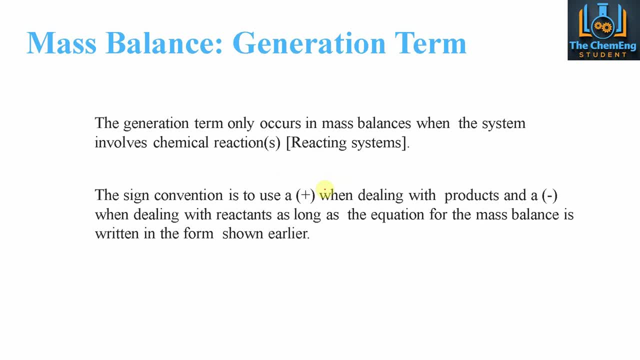 there was a plus and a minus at the generation term in the general balance. Now the plus is when we deal with products and the negative is when we deal with reactants. because if we consider the generation, if we have a negative, then that means that we are losing the component. 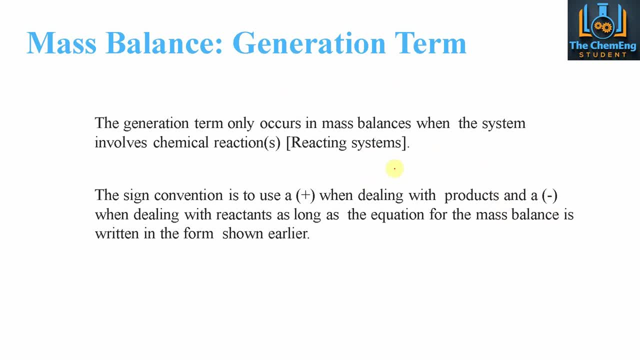 So the reactant will of course get less as the reaction proceeds, and then the product will increase in value as the reaction proceeds. Now, normally what we do is we model around one of the reactants, Some things. we model around the limiting reactant and that will tell us the minimum value. 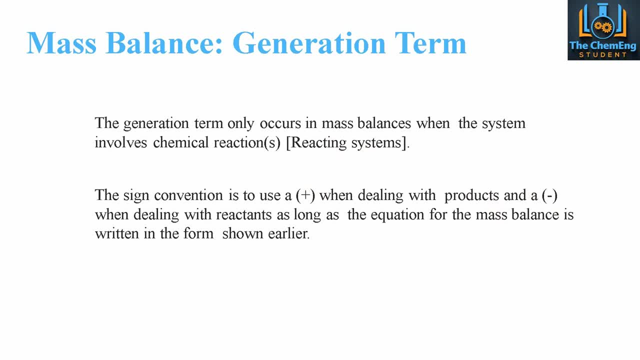 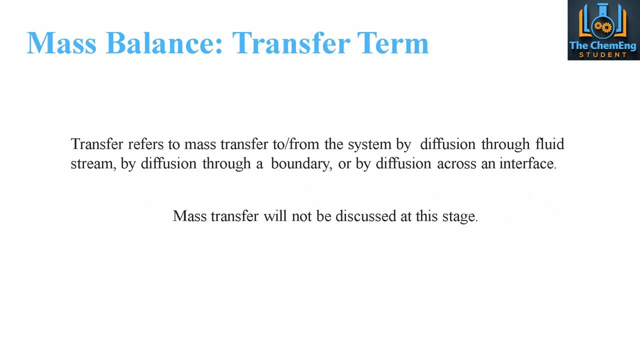 that we can achieve in terms of the mass of the products or any other variable of interest. Now the transfer term. It refers to mass transfer to and from the system by diffusion through fluid steam, by diffusion through a boundary layer or by diffusion across an interface. Now mass transfer. in this lesson, 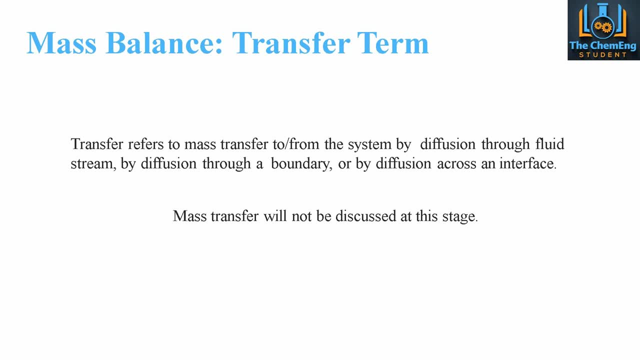 won't be discussed. however, we do have a dedicated course that considers mass transfer, and we also cover mass transfer in our mass and energy balance course. So if you want to know more about the depth analysis on mass transfer, please do check that one out. I'll put a link in the description. 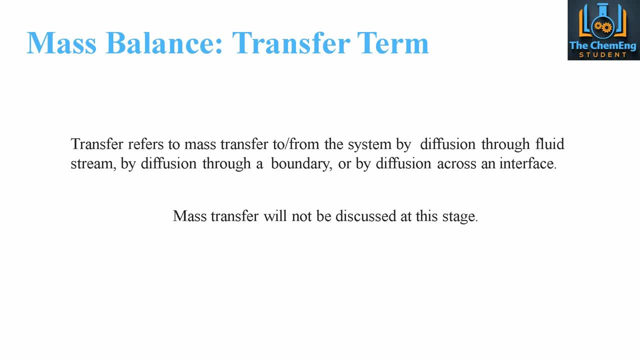 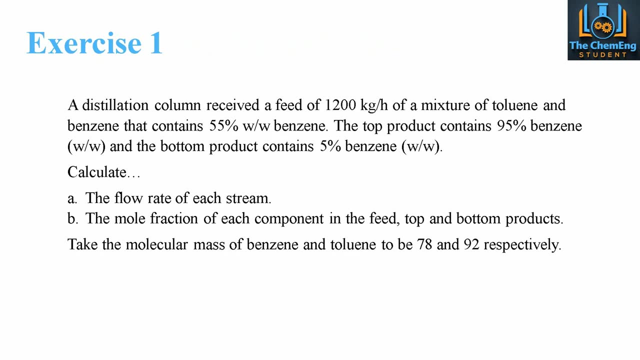 on the website, where you can find more details about us there. So if we look at a working exercise now, this is for non-reacting systems. It says we have a distillation column which receives a feed of 1200 kilograms an hour, and it's a mixture of toluene and benzene that contains 55 percent weight. 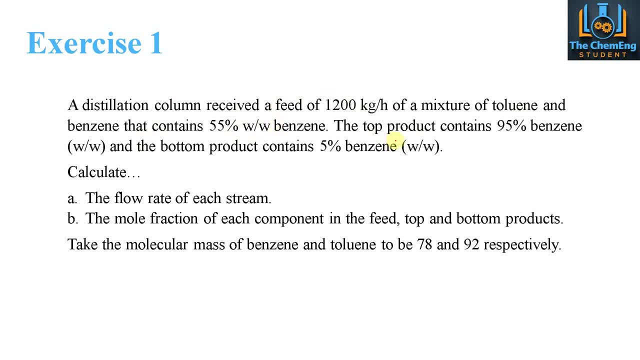 so that is in the feed. Now. the top product contains 95 percent benzene weight per weight and the bottom product contains five percent benzene weight for weight. Now we need to calculate the flow rate of each of the streams and then the mole fraction of each of the components within the 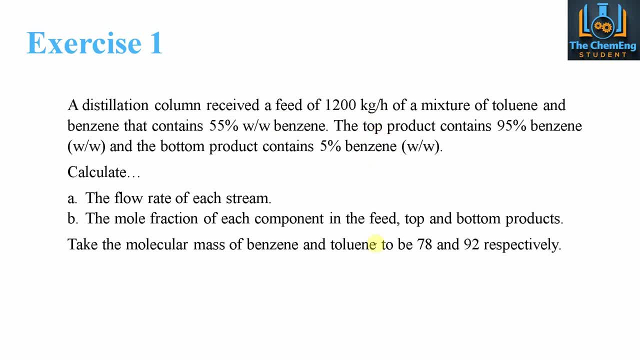 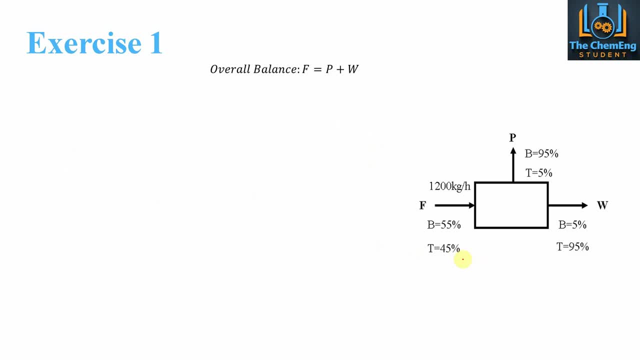 feed The top product and the bottom product, and it gives us our molecular masses of benzene to be 78 and toluene to be 92. So the first thing that we'll do is we will express the information that we were given on a block diagram. 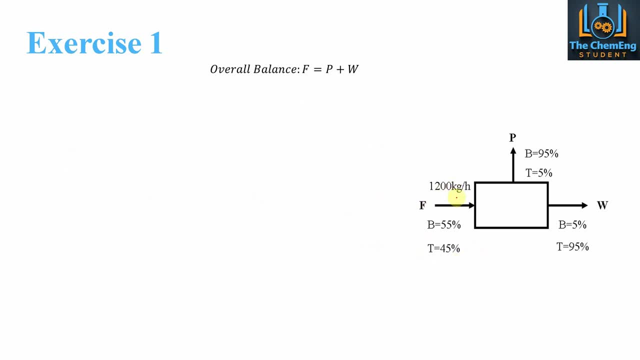 So we have our feed coming in, so we have a flow rate of 1200 and we know the composition of the feed. Now, B denotes benzene and T denotes toluene. so we know that at the top product we have 95 benzene, five percent toluene- that would give us our hundred percent. and then at the bottom product we 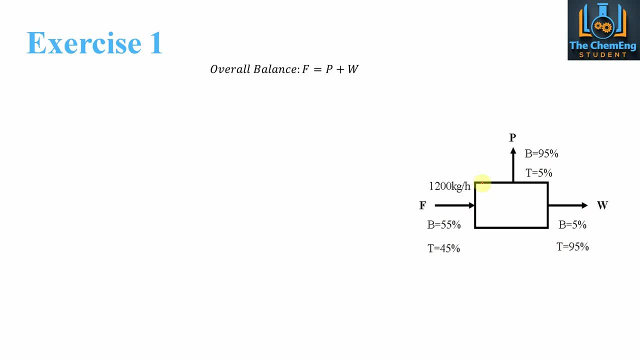 have five percent benzene and 95 percent toluene. Now the overall balance must be: what comes into the system is equal to what leaves the system. So the feed is equal to p plus w. so that means that the values of p and w must add up in terms of flow. 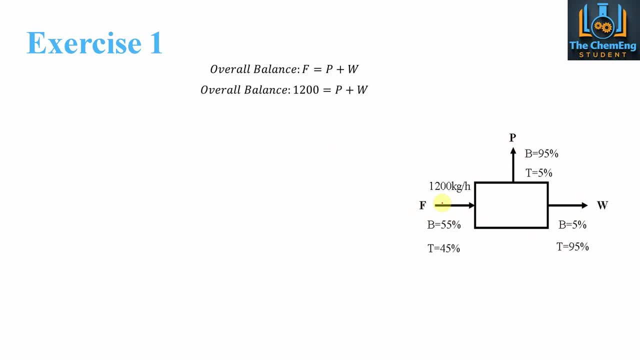 rate to the value of f. Now what we can then say is: once we have this equation sorted, we then need to perform a component balance. Now, we'll balance benzene over the other components, the entire system. now we know that benzene is 55%, so we'll do 0.55. 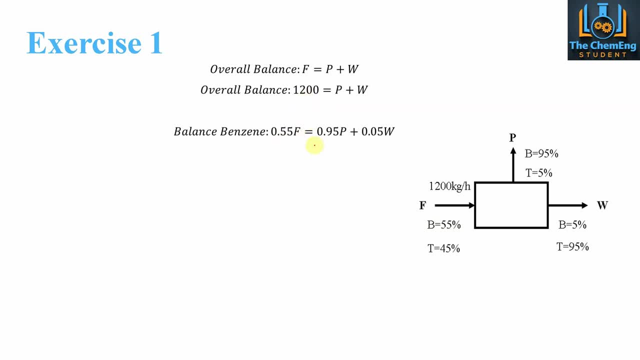 multiplied by the feet, now we know the feed is 1200 and that's equal to there is 0.95 and the top product plus 0.05 and the bottom product. now when we substitute in the value of F, we get 660 as the flow rate of benzene. now we can. 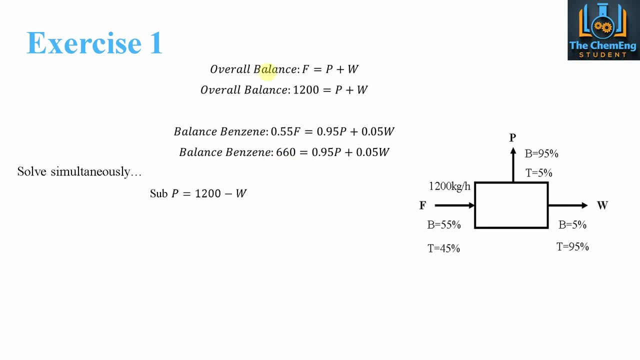 solve using simultaneous equations. so we can rearrange this for P. ultimately you could do it for W as well, but here we're going to do it for P. so we know that P is equal to 1200 minus W, so we can substitute that in here and find the 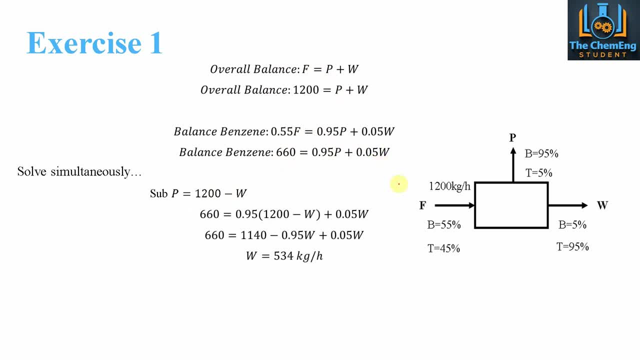 value of W. so in doing so, we find that W has a flow rate of 534 kilograms an hour. so therefore we can work out what P is, because that's of course going to be 1200 minus 534, so that gives us a P value of 666 kilograms per hour. now the moles is the triangle that you sometimes 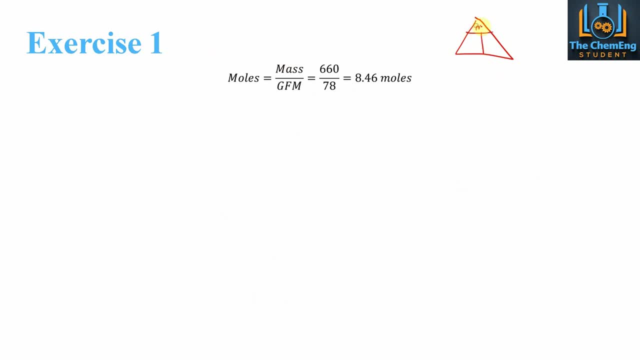 see in your chemistry classes is seen like this: so this is the mass, this is the moles and this is the GFM. so this is the gram formula mass or molecular mass. so by rearranging this, we know that the moles is equal to the mass divided by the GFM. so if we do this in terms of a benzene, 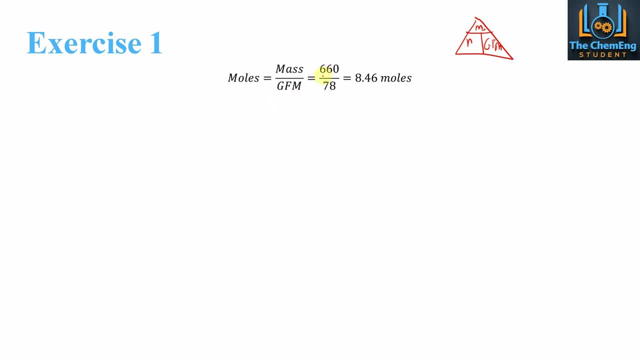 then this is for the top product in benzene, so we have 8.46 moles. now this is just a sample calculation in order to show how we work out the fraction, or the mole fraction, sorry, of our system. so this is for the top product, so we know. 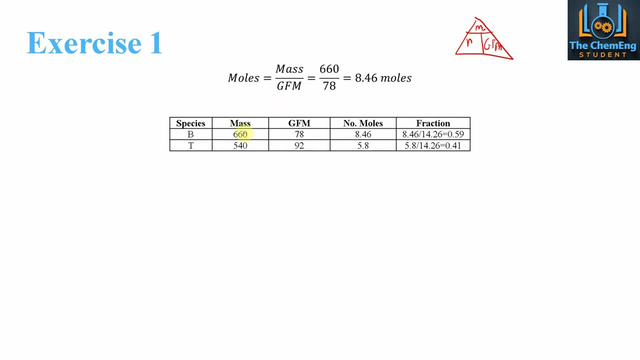 that if we balance a species, a, B, then our mass is 660, we have a GFM and we have a number of moles. then what we can do is do the same thing for toluene. so that would be 540 divided by 92. that would give us a number of moles of 5.8. 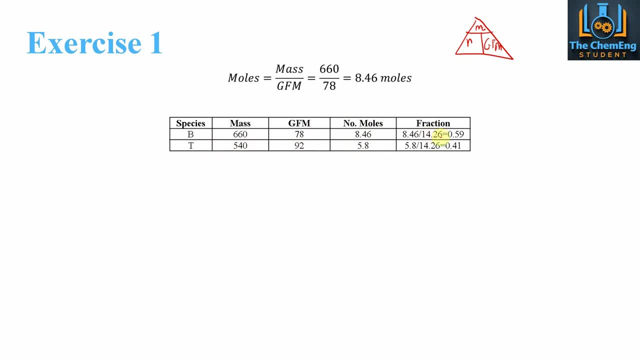 now, if we add these values together, we get 14.26. so then we divide our respective moles by the total, and that will give us 59 percent benzene and 41% toluene. Now for the top product. the total mass was 666 kilograms an hour, So what we can. 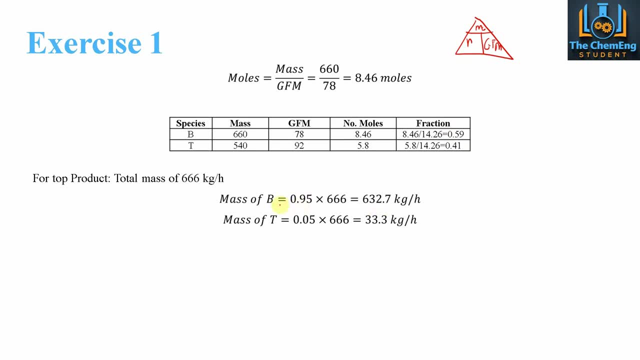 then do is say that we have 95 of benzene at the top. so we multiply that by 666, that will give us 632.7. and then we can do: 0.05 multiplied by the flow rate will give us 33.3.. 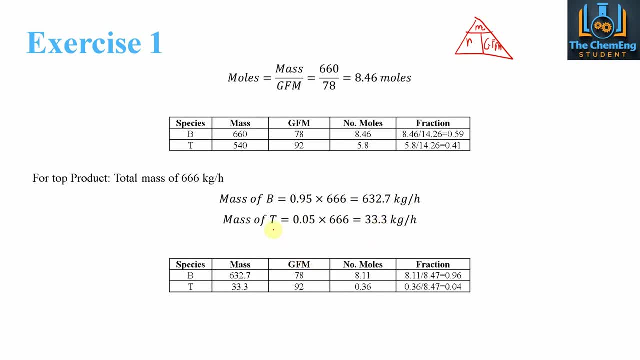 So then we can perform the same system again for the top product. so we know the mass flow rates, we know the GFMs, we can calculate the number of moles using that equation, and then we work out the total- so that would be 8.47- and then divide the respective moles. we get 0.96 and 0.04.. 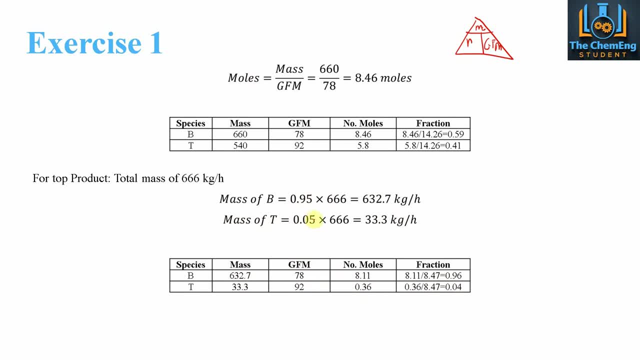 So they are very, very close to the assumed values, which makes sense. if we got a value here of 80 odd, we would get 0.96 and 0.04.. So we can calculate the number of moles using that equation and then then there's probably an error that we've done somewhere. we've maybe used the wrong flow rate. 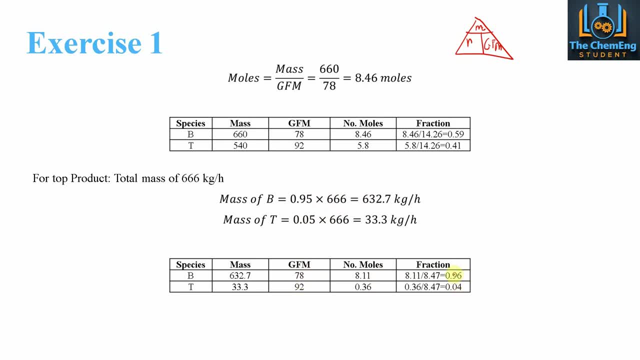 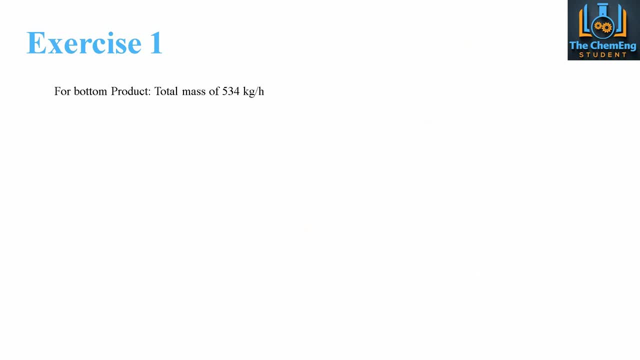 or we've maybe got the GFMs mixed up so they should be around what the estimated values were in the question. Now for the bottom product, the total mass. we were told flow rate was 534 kilograms per hour. so we do the same thing. we multiply 0.05 and 0.95 for benzene and toluene. 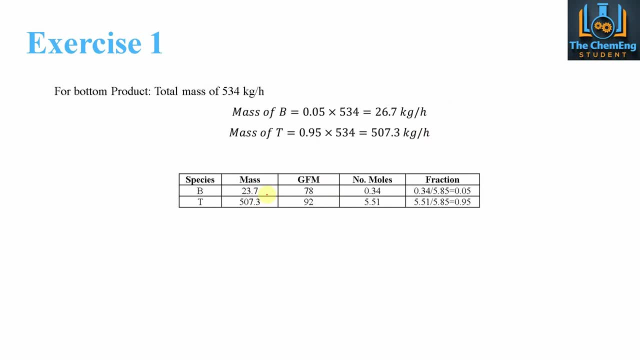 respectively. So then when we substitute in our table mass GFM moles again, we see that we get the exact values of 0.95 and 0.05.. So that just proves that our mole fraction is weight per weight what it said in the question. So that's the end of this lesson. thanks for watching. hopefully this has. 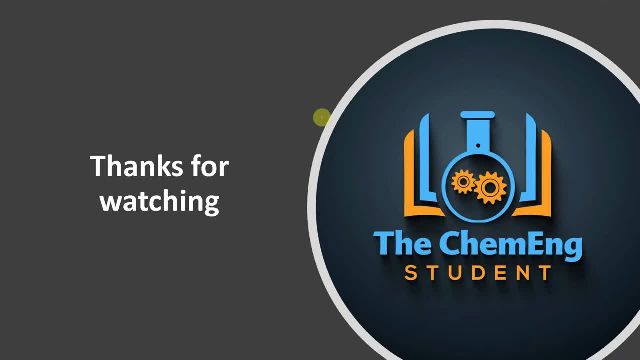 enhanced your understanding of mass balances. Please leave a like and subscribe to the channel. Leave any comments in the comment section below and we hope to see you in another video.